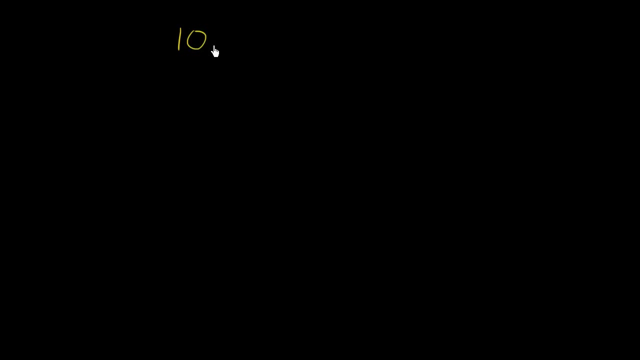 Let's say that I'm working in a restaurant and I'm making $10 per hour, But on top of my hourly wage I also get tips each hour. So this entire expression- you can view this as how much I might make in a given hour. 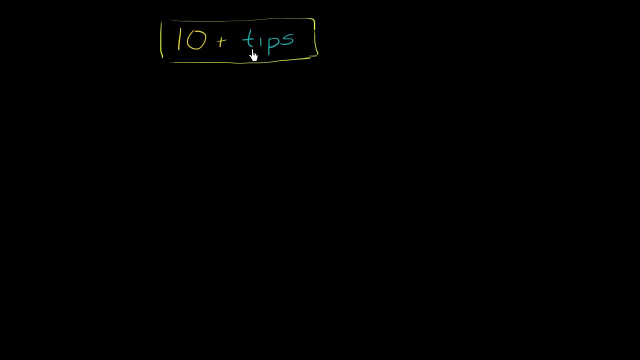 Now you might also realize that the number of tips or the amount of tips I might make in an hour can change dramatically from hour to hour. It can vary One hour, it might be lunchtime. get a lot of tips. People might get some big ticket items. 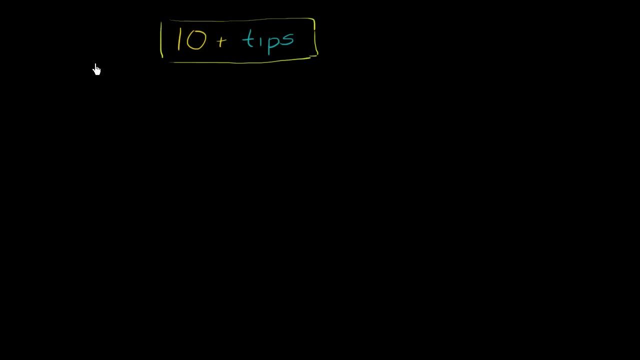 The next hour I might not have any customers And then my tips might be really low. So the tips part right over here. we consider that the entire word. we consider that to be a variable From scenario to scenario. it can change. 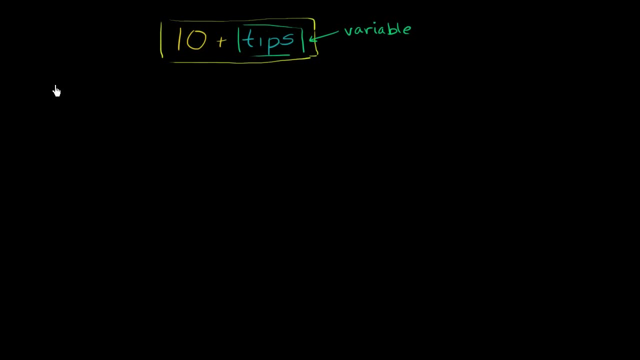 So, for example, in one scenario- maybe it's lunchtime- I'm getting really big tips. So tips is equal to, let's say it's equal to $30.. And so the total amount I might make in that hour is going to. 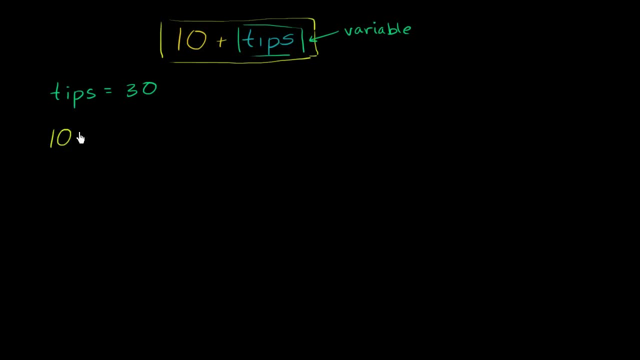 we can go back to this expression right over here. It's going to be 10, plus instead of writing tips here, I'll write 30, because that's what my tips are in that hour, And so that is going to be equal to 40.. 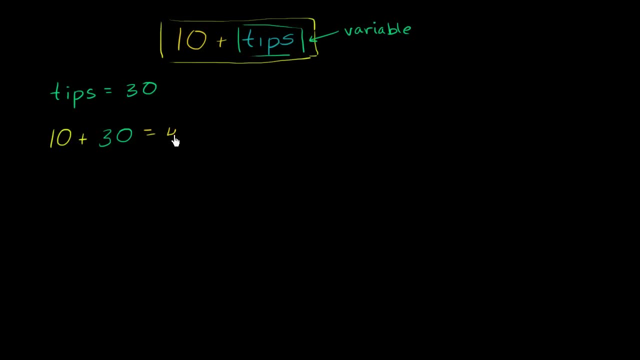 Let me do it in that yellow color. It's going to be equal to $40.. But let's say right after that the restaurant slows down, We're out of the lunch hour for whatever reason. Maybe the restaurant next door has a big sale or something. 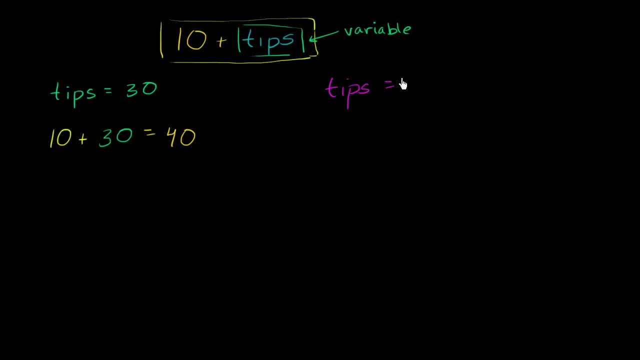 And so the next hour my tips go down dramatically. My tips go down to $5.. $5 for that hour- Now I go back to this expression. The total I make is my hourly wage plus the $5 in tips, which is equal to $15.. 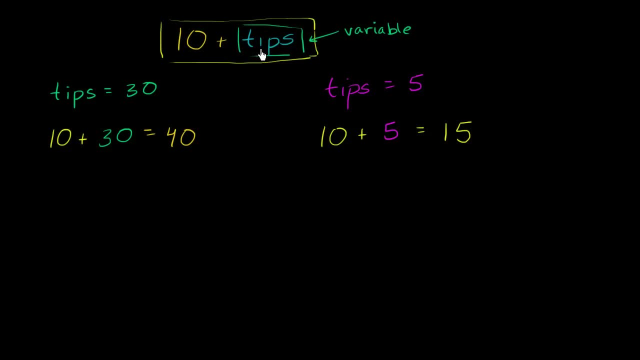 As you see, this entire expression, the 10 plus tips. it changed depending on what the value of the variable tips is. Now you won't see whole words typically used in algebra as variables. We get lazy, And so instead we tend to use just. 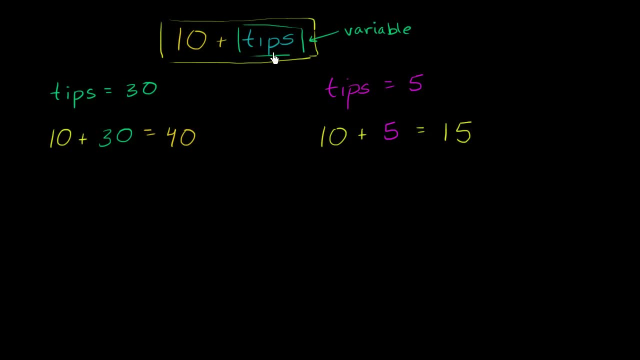 easier to write symbols, And so, in this context, instead of writing tips, maybe we could have just written 10 plus t, where t represents the tips that we get in an hour, And so then we would say: OK, what happens when t is equal to 30?? 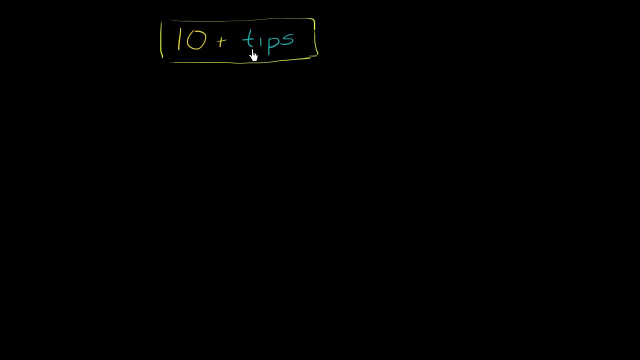 Now you might also realize that the number of tips or the amount of tips I might make in an hour can change dramatically from hour to hour. It can vary One hour, it might be lunchtime. get a lot of tips. People might get some big ticket items. 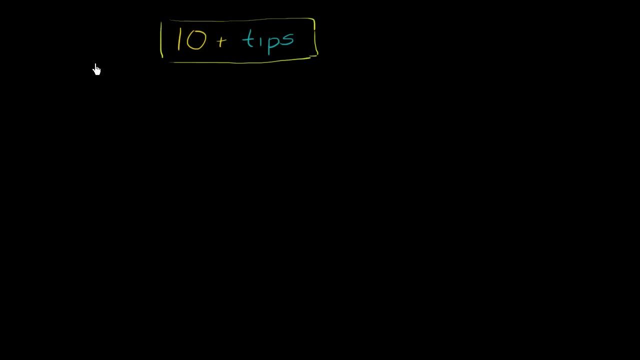 The next hour I might not have any customers And then my tips might be really low. So the tips part right over here. we consider that the entire word. we consider that to be a variable From scenario to scenario. it can change. 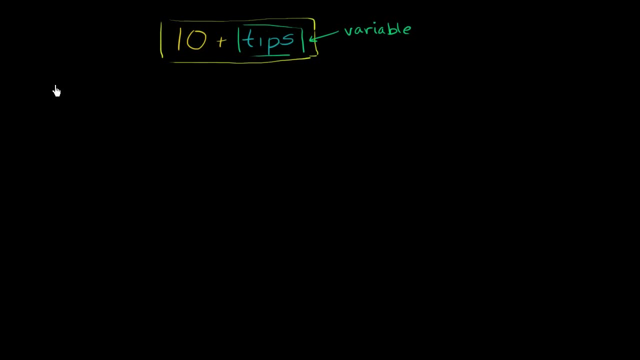 So, for example, in one scenario- maybe it's lunchtime- I'm getting really big tips. So tips is equal to, let's say it's equal to $30.. And so the total amount I might make in that hour is going to. 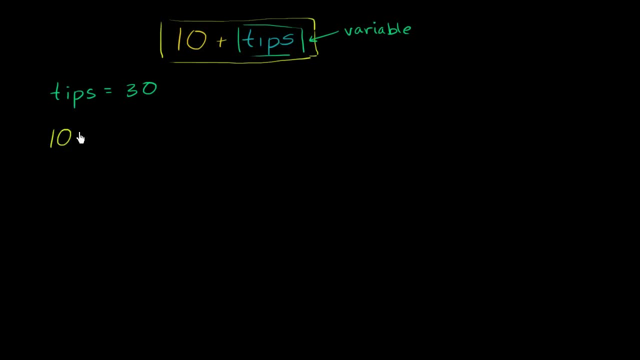 we can go back to this expression right over here. It's going to be 10, plus instead of writing tips here, I'll write 30, because that's what my tips are in that hour, And so that is going to be equal to 40.. 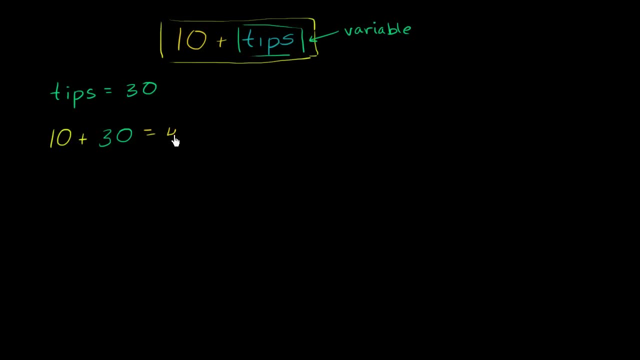 Let me do it in that yellow color. It's going to be equal to $40.. But let's say right after that the restaurant slows down, We're out of the lunch hour for whatever reason. Maybe the restaurant next door has a big sale or something. 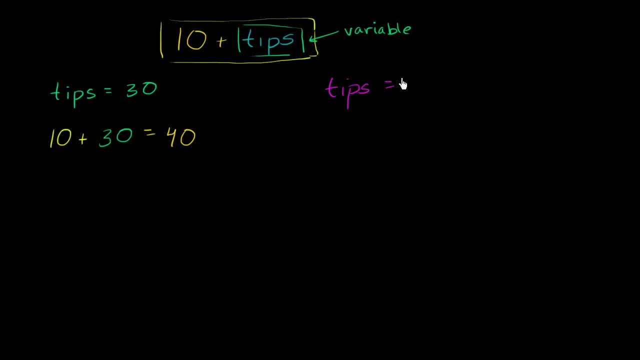 And so the next hour my tips go down dramatically. My tips go down to $5.. $5 for that hour- Now I go back to this expression. The total I make is my hourly wage plus the $5 in tips, which is equal to $15.. 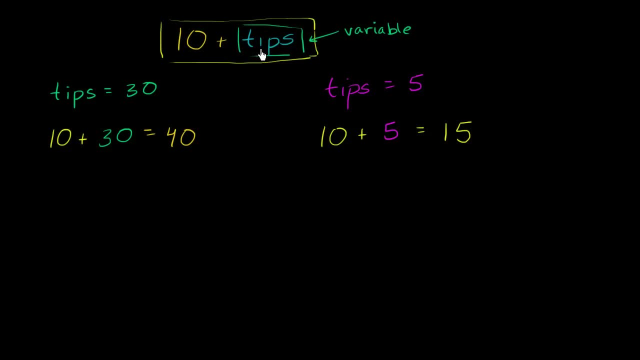 As you see, this entire expression, the 10 plus tips. it changed depending on what the value of the variable tips is. Now you won't see whole words typically used in algebra as variables. We get lazy, And so instead we tend to use just. 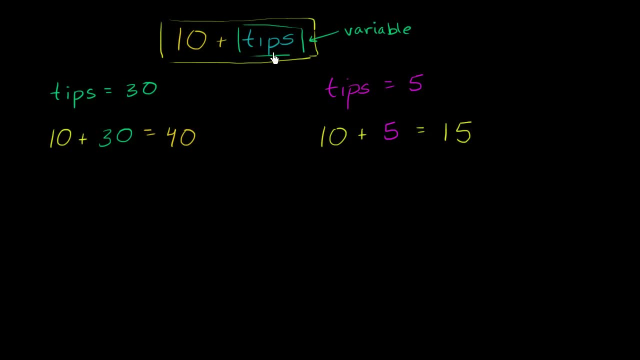 easier to write symbols, And so, in this context, instead of writing tips, maybe we could have just written 10 plus t, where t represents the tips that we get in an hour, And so then we would say: OK, what happens when t is equal to 30?? 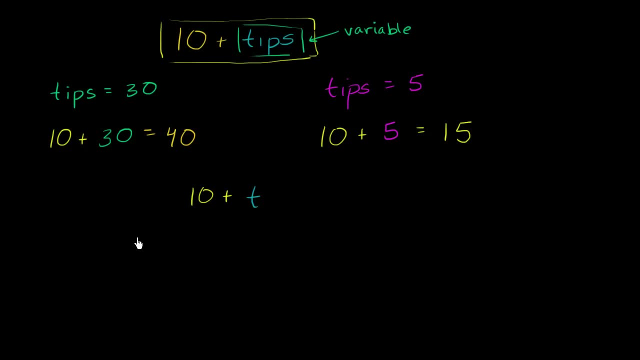 Well, if t is equal to 30, then we'd have let me write: so what happens when t is equal to 30?? Well then we have a situation: t is equal to 30. This evaluates to 10 plus 30,, which would be 40..